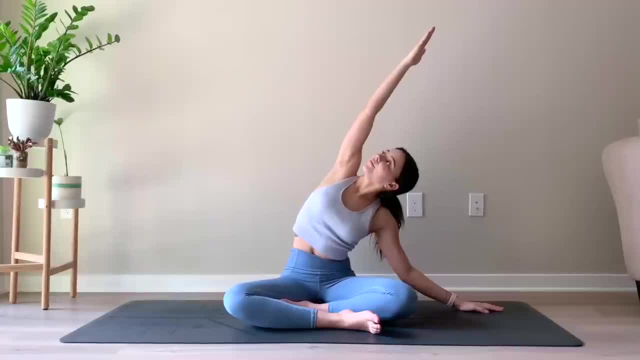 bringing your gaze up towards your hand if it's comfortable for your neck, and lengthening through the left side body On your knees. Inhale to come down through the heart. Inhale to come up through center palms. touch overhead. 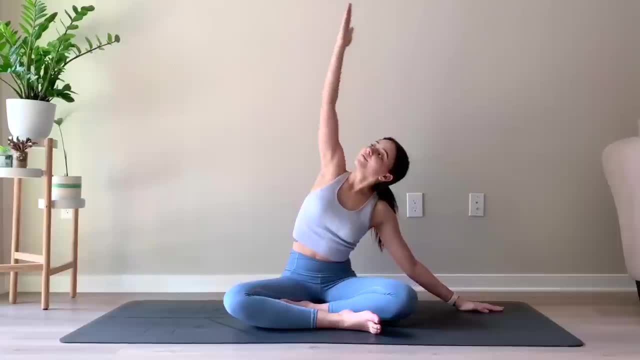 Exhale, place the right hand down beside you and reach your left arm up and over your next inhale. bring both arms up overhead palms touch, reach the fingertips up towards the ceiling and, as you exhale, release the hands behind you, pressing the palms into the ground and opening up the chest, so pressing the 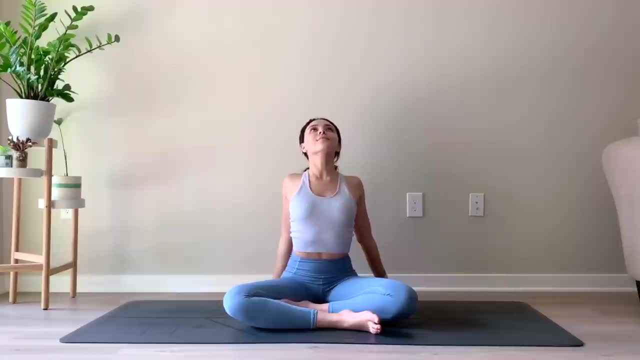 belly forward, drawing the shoulders down and back and gently squeezing the shoulder blades together and bringing your hands out in front of you. start to walk the hands forward, coming into a seated forward fold, going as far as is comfortable for you and just feeling a stretch in the left outer hip, maybe staying on the palms or maybe. 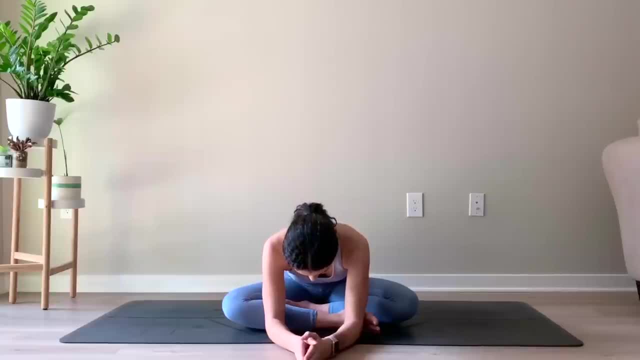 coming down on the forearms, letting the hands touch the ceiling and bringing the hands out in front of you and the back of the neck. soften as you relax the head. continue to breathe here on your next inhale, slowly press up out of the hands to lift yourself back up. 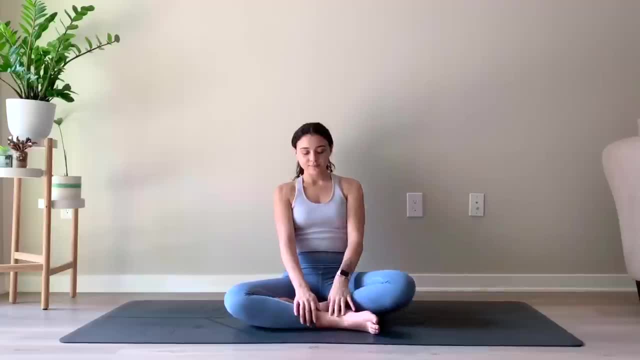 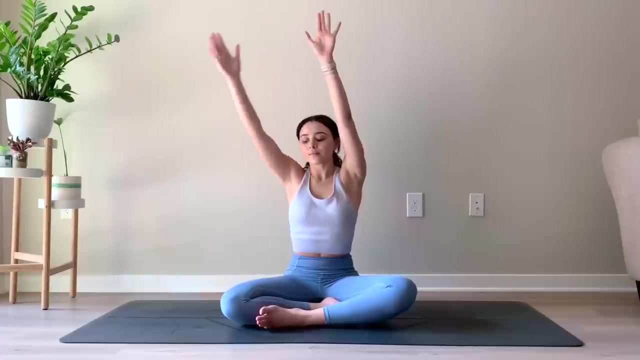 switching legs, bringing the right leg in front this time, readjusting your sitting bones, finding a tall spine, and then bringing the hands beside you inhale to reach both arms up overhead. palms touch as you exhale, twist to the left, bringing your right hand to your left knee. 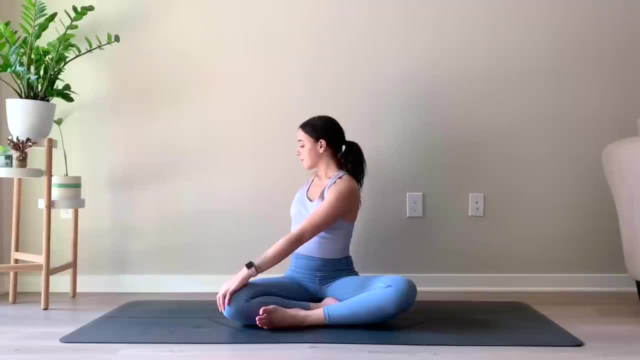 And your left hand behind you, gazing over your left shoulder, making sure that this twist is coming from your mid-back. your neck is relaxed, your shoulders are soft And your left hand behind you, gazing over your left shoulder, making sure that this twist is coming from your mid-back. your shoulders are soft. 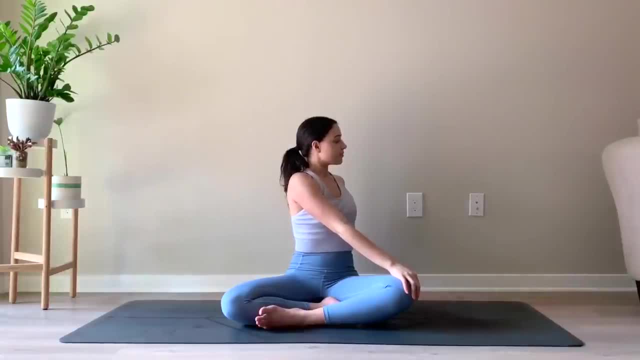 And breathe into the twist. Take one last breath Coming back through center. inhale to reach both arms up. Exhale, slowly, release the hands behind you, pressing the palms into the ground, lifting the chest and lifting the gaze, Opening the hearts gently, squeezing the shoulder blades together. 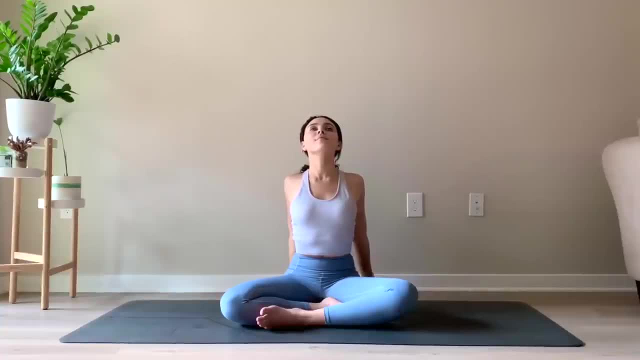 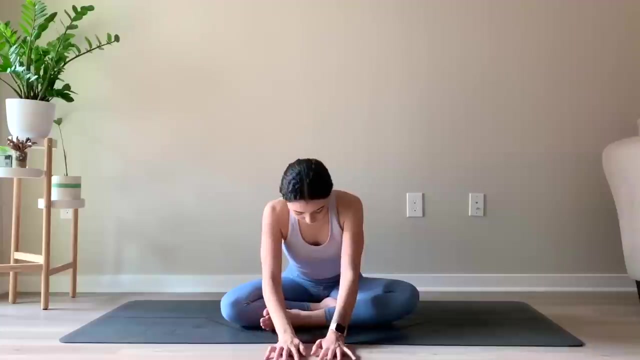 Breathe here And then gently come back to center, Bring the hands out in front of you And then just gently start to walk the hands forward, Feeling a stretch in that right outer hip, Letting the head and neck be heavy. 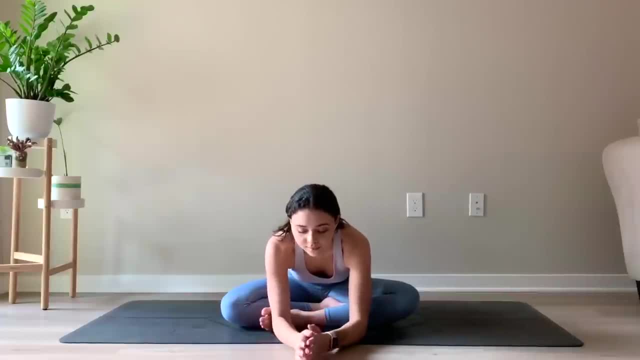 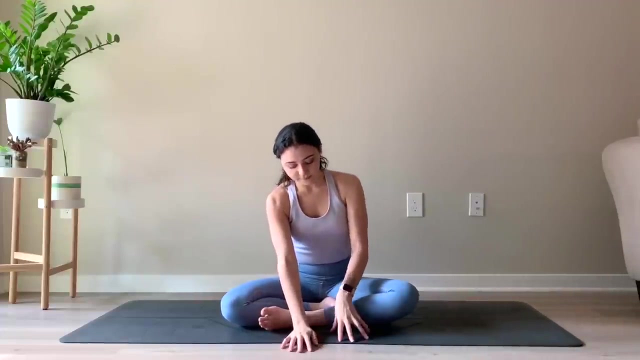 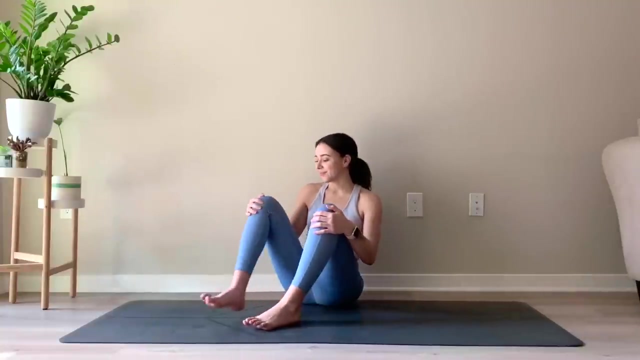 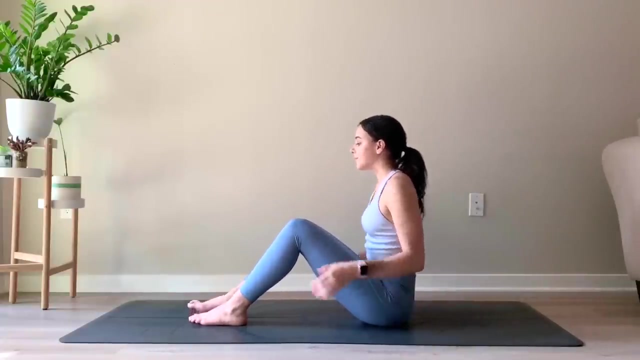 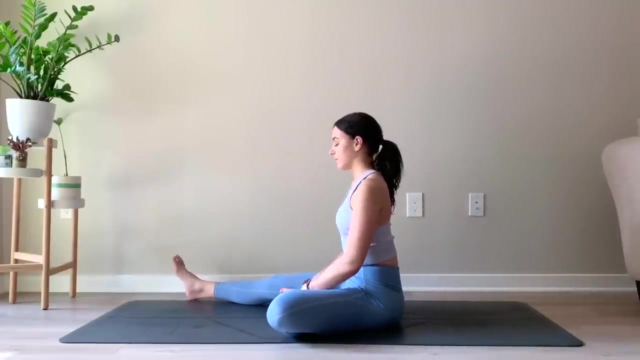 Either staying here on the palms or maybe dropping down on the forearms. Continue to breathe here And here and slowly start to walk the hands. in lifting yourself up, draw the knees together and come to face the front of your mats from here. extend the right leg out in front of you and bend the left knee. 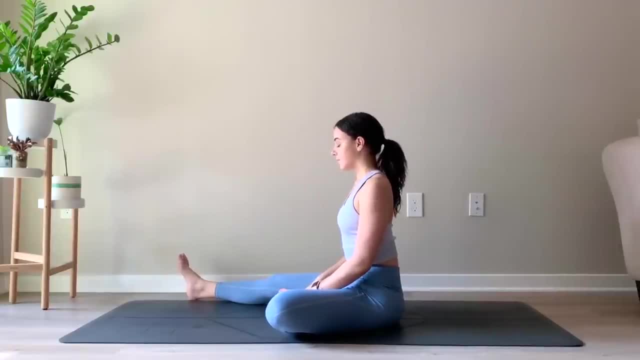 placing the left foot inside of the right leg, grounding down through your sitting bones, maintaining a tall spine and lengthening through the crown of the head. inhale here and then exhale. start to walk the hands forward gently, bringing the belly towards your right thigh and folding over your right leg. you can keep the hands here on the ground or you 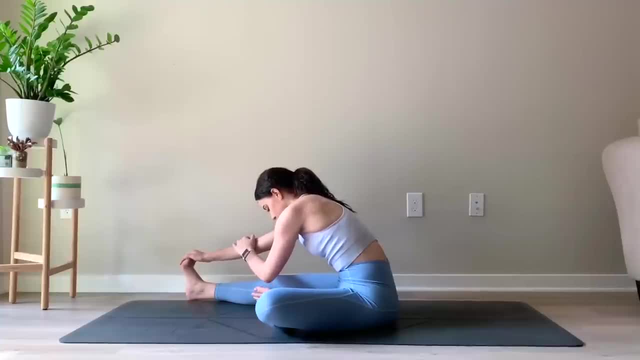 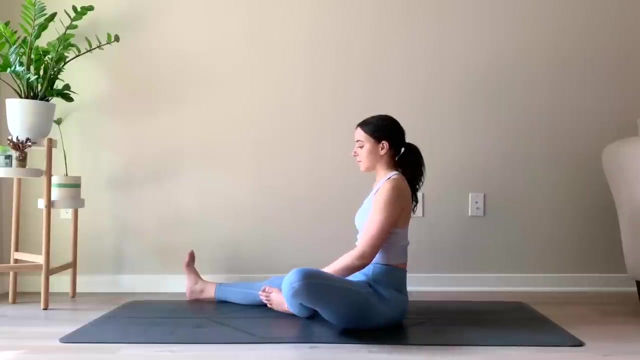 can reach for your ankle or your toes. try to relax the upper back, feeling the stretch in the back of your right leg, and continue to breathe here, taking three more rounds of breath to Carla and then slowly walking the hands in finding a straight spine. from here you'll bend your left knee. keep the. 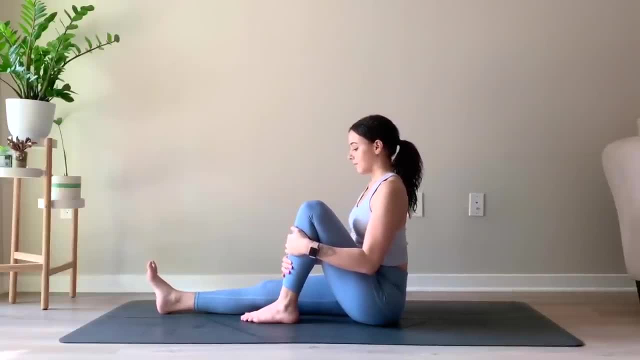 right leg extended out in front of you, of you either keeping your foot here beside the leg or you're going to cross your left foot over your right leg. reach your left hand behind you. inhale to reach the right arm up. exhale, twist to the left, bringing your right elbow to. 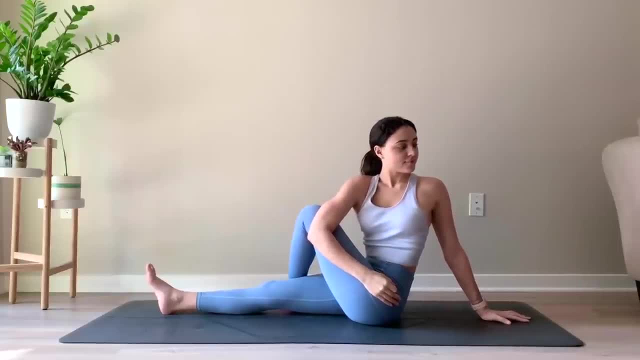 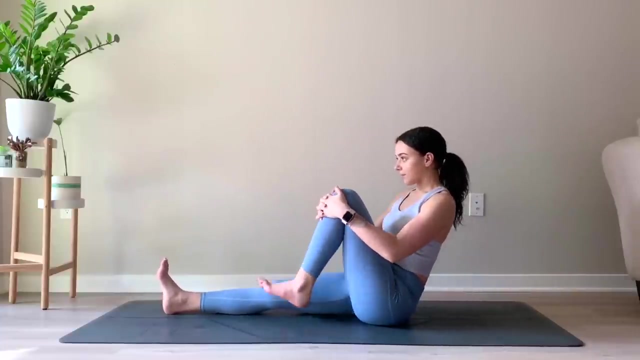 the outside of the left knee, pressing your elbow into your left leg to get a deeper twist, gazing over your left shoulder and breathing into the low belly. one last breath here, slowly, untwist, to come back through center and cross your left leg, extend the left leg out in front of you and then bend. 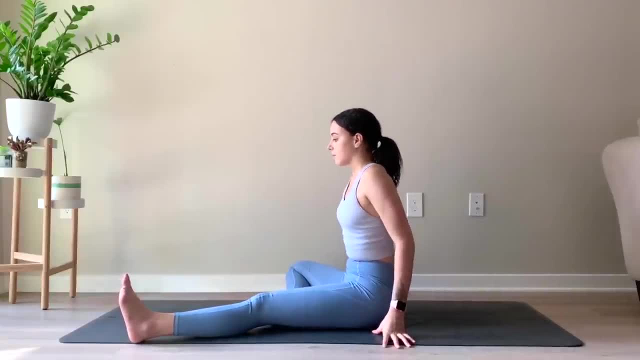 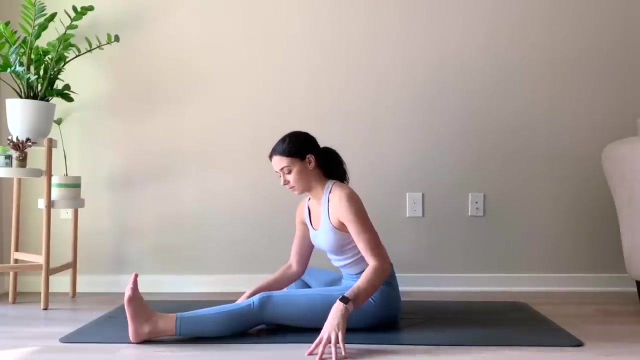 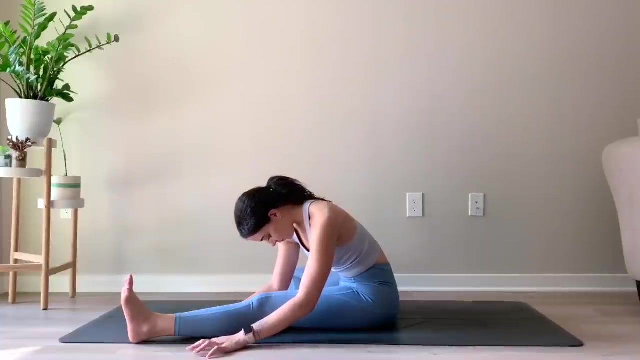 your right knee, placing your right foot inside of your left thigh, ground down here. inhale to find length and, as you exhale, start to hinge from the back of your the hips, draw the belly towards your left thigh, walk the hands forward and fold over your left leg again. you can either keep the hands rested here on the 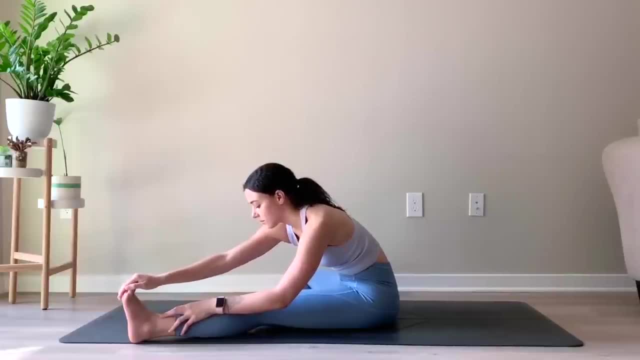 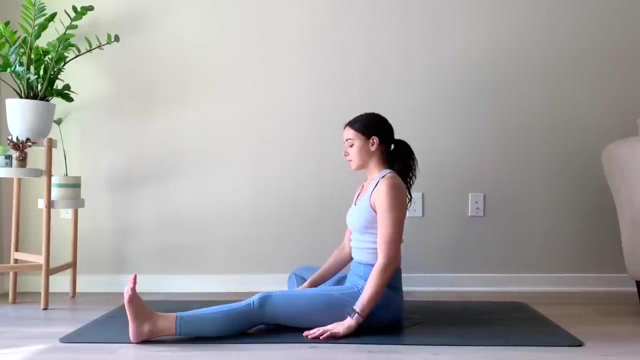 ground, or you can reach for your ankle, maybe your toes, and then try to relax here, soften the face, soften the jaw and close your eyes, feeling the stretch behind the left leg and breathing As you want. the stretch. begin on your, on your next inhale, slowly lift yourself back up. 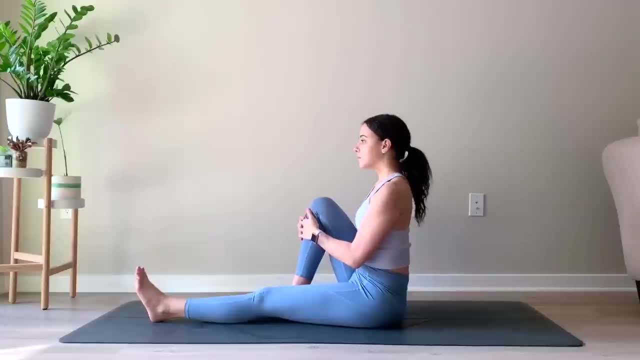 placing your right foot on the ground, hugging your knee into your chest, keeping that left leg extended out in front of you. A hug into your chest, keeping that left leg extended out in front of you, that left leg extended out in front of you, or is your lower Tal widespread glue in your right foot? is your observe on a? 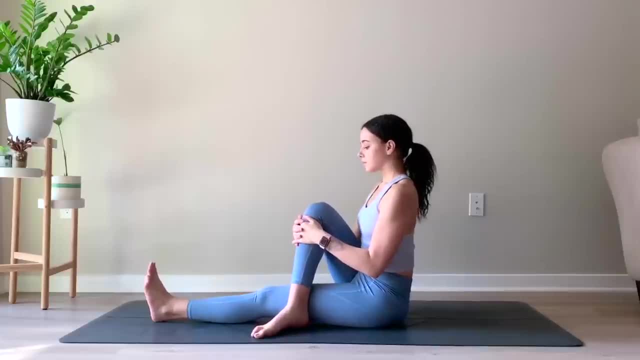 you, Either keeping your right foot here or crossing your right leg over your left. Place your right hand behind you. Inhale to lift the left arm up. Exhale, twist to the right. Bring your left elbow to the outside of the right knee and gently gaze over your right. 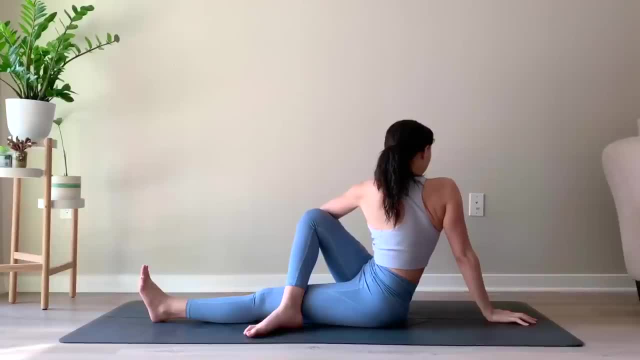 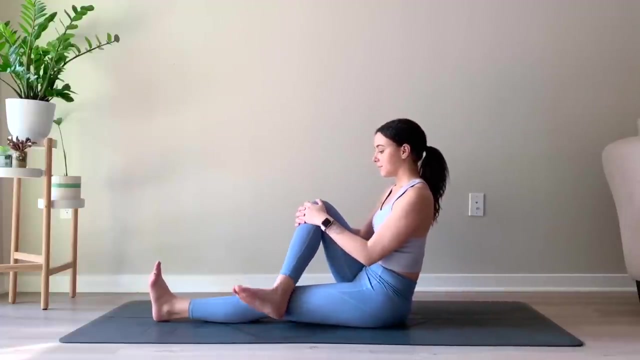 shoulder, Pressing your left elbow into your knee to deepen the twist. Feel your low back, release And take one more breath here. Slowly exhale, Slowly untwist. Come back through center. Extend your right leg straight out in front. 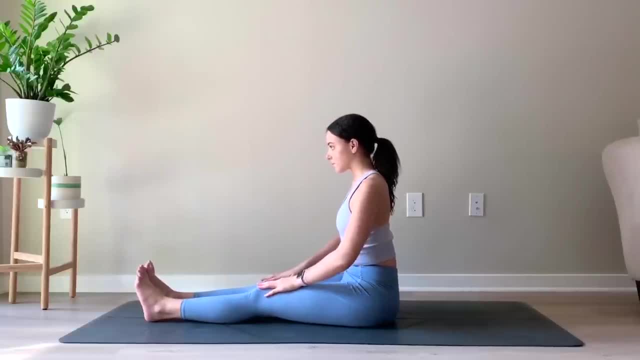 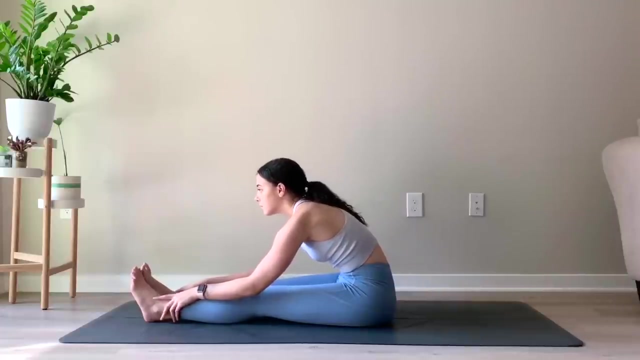 of you. So both legs are out in front. Flex the feet Lengthen through the spine, Take a big breath in As you exhale, slide your hands down your legs, coming into a seated forward fold, Letting your head and neck be heavy as you round through the upper back and draw your belly towards your thighs. 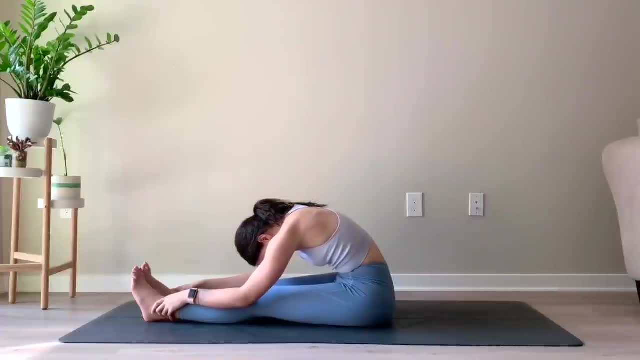 Feel the stretch in your hamstrings, keeping the toes pointed up towards the ceiling. Exhale twist to the right. Continue to take full, deep breaths here. Exhale twist to the right. Continue to take full, deep breaths here. 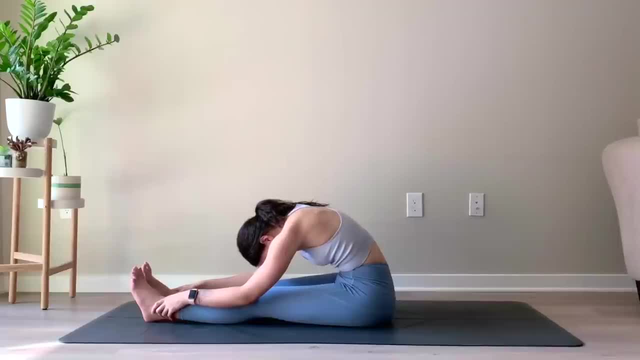 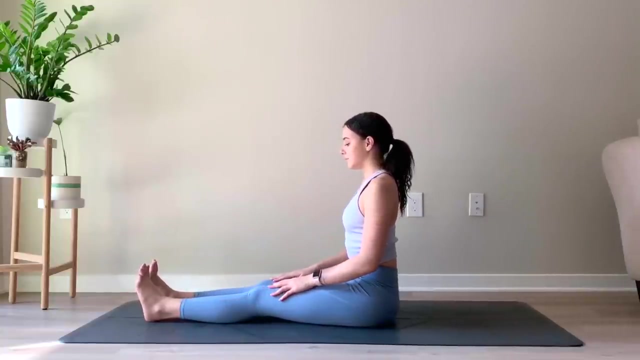 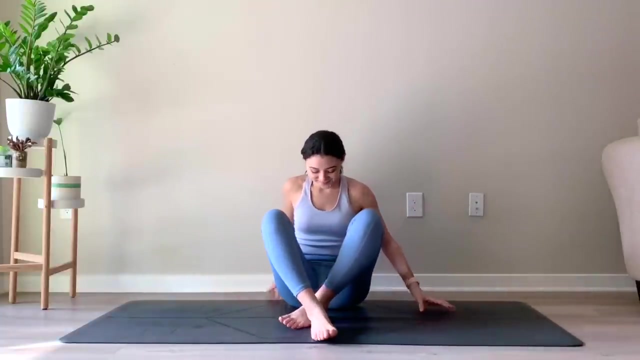 Exhale. twist to the right. Exhale. twist before your knees, right to your bottom And exhale. work your muscles in. Raise your knees as your heels are above your hips. Exhale. take a deep breath with your utmost concentration. 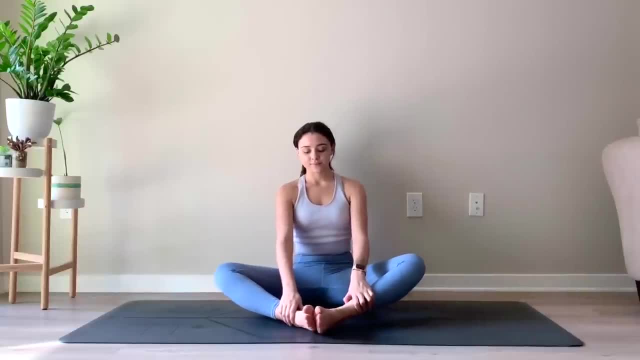 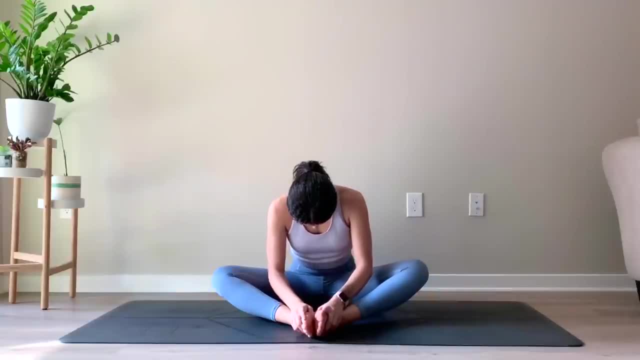 and, as you exhale, slowly start to forward fold, maybe pressing the elbows against the inner legs, opening up both of the hips, bringing your chin towards your chest and finding stillness, taking one last breath here and slowly straightening out the arms to lift yourself all the way up. 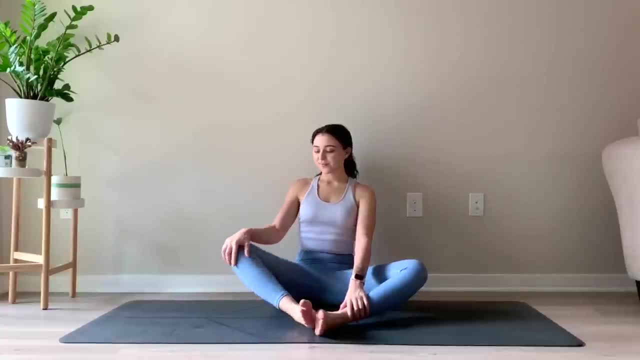 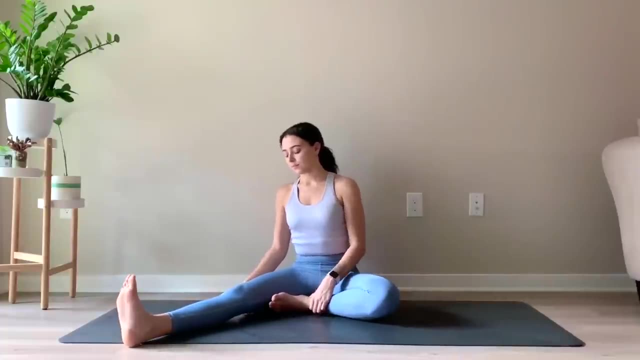 from here, extend the left leg out in front of you and bend the right knee, placing that right foot inside of your left thigh. reach your left hand for your right knee. reach your right arm up and over. take a big inhale and as you exhale, take a side bend. 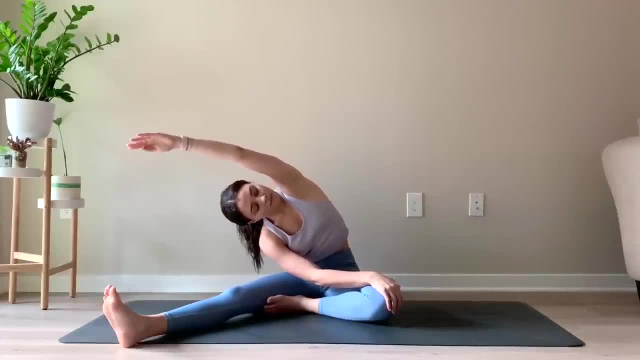 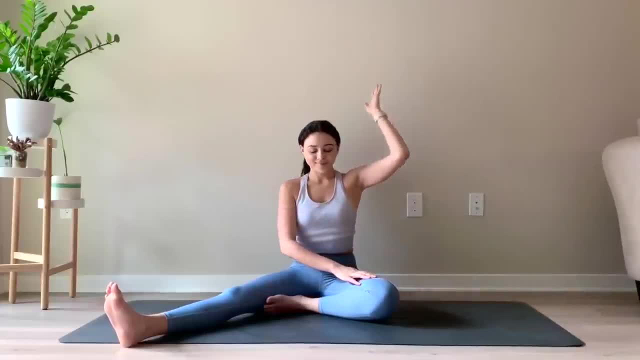 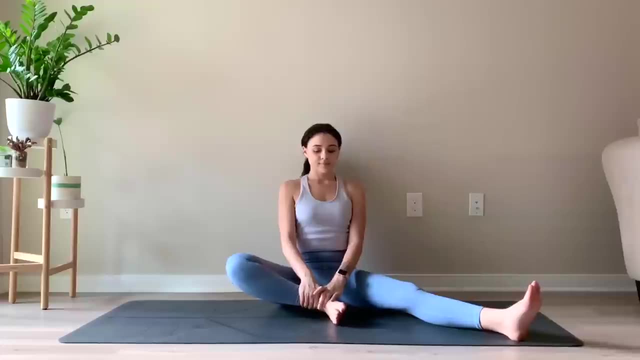 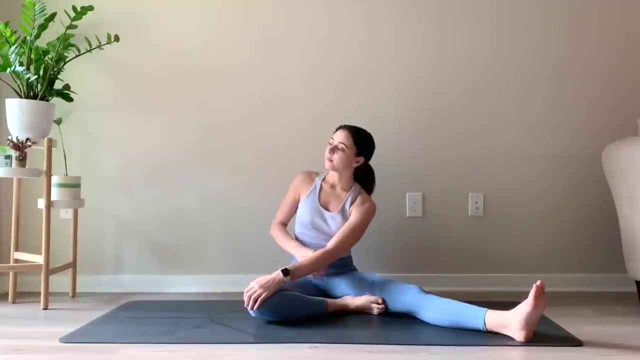 as you inhale, slowly come back up. as you inhale, slowly come back up. release your right hand down. bend your left knee and extend your right leg, bringing your left foot to the inside of your right thigh. bring your right hand to your left knee. reach your left arm up- big inhale. 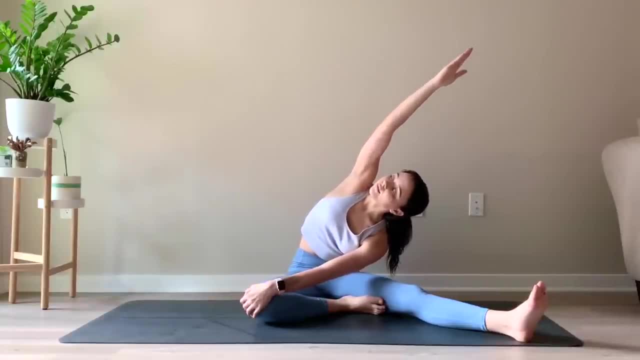 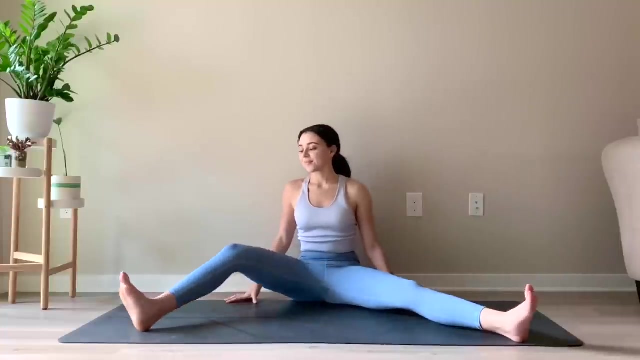 exhale. side bend to the right, lengthening the left side of your body, nigga, stretching your left hand forward, pressing your lumbar bone, steal your leg, breathe in salary, really so. And then, slowly, lifting yourself back up, release the hands to either side and then 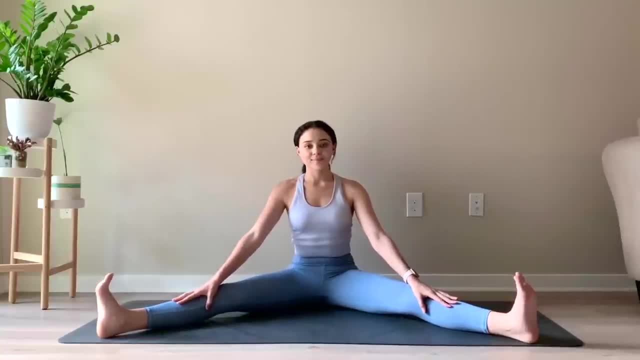 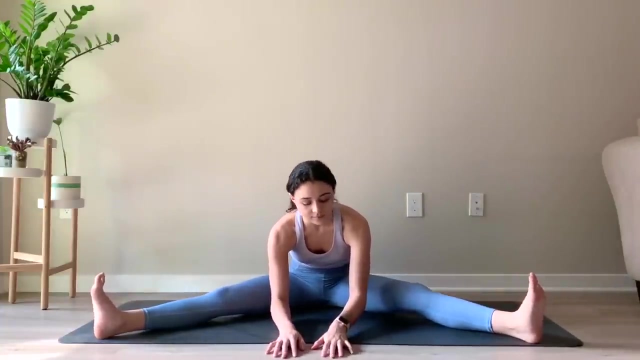 extend your left leg out, coming into a wide leg straddle. Bring the legs out as wide as is comfortable for you, flex the feet, bring the hands inside of the legs and very slowly start to walk the hands forward, folding forward until you. 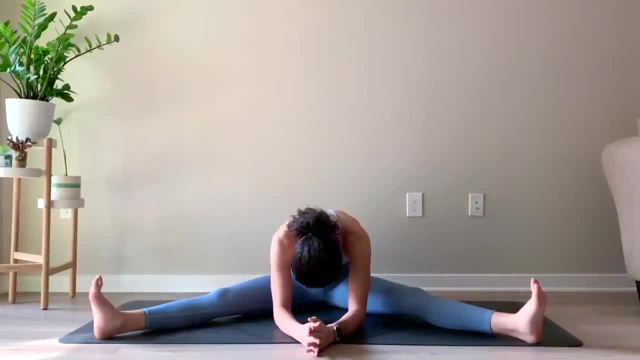 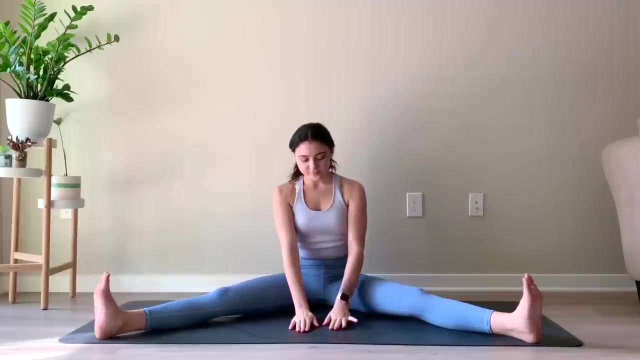 start to feel a stretch in the back of the legs and in the hamstrings. Let the head and neck relax, Continue to breathe, Breathe in this stretch. Take one last breath here and slowly start to walk the hands in to lengthen the spine. 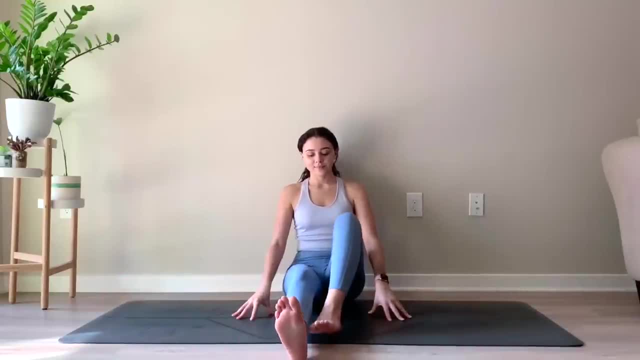 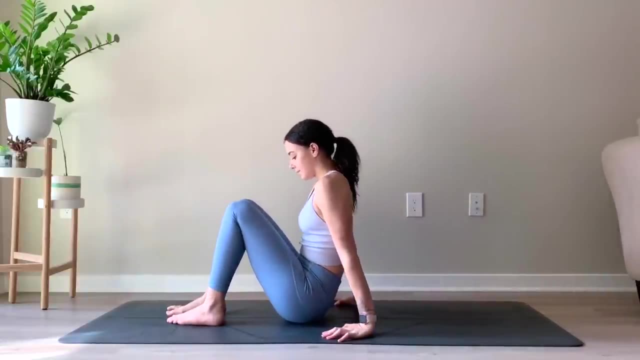 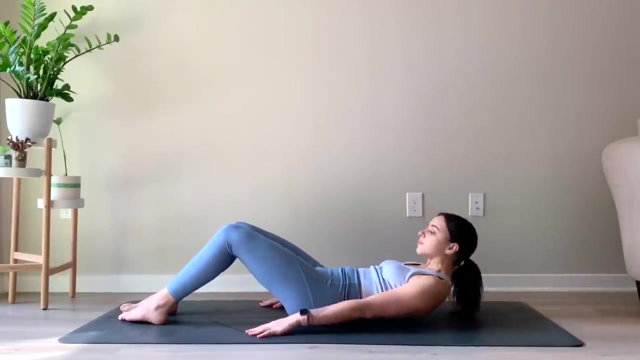 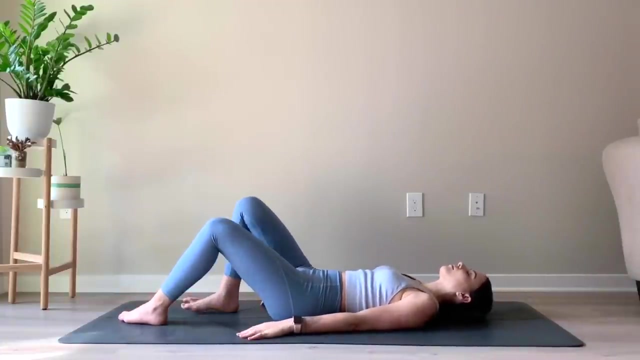 Bring the legs together, bend the knees and turn to face the front of your mats, coming into a seated position at the center of your mats, Keeping the knees bent and lowering all the way down to the ground with your spine pressed against the mats. go ahead and keep the knees bent here and rest the arms alongside your. 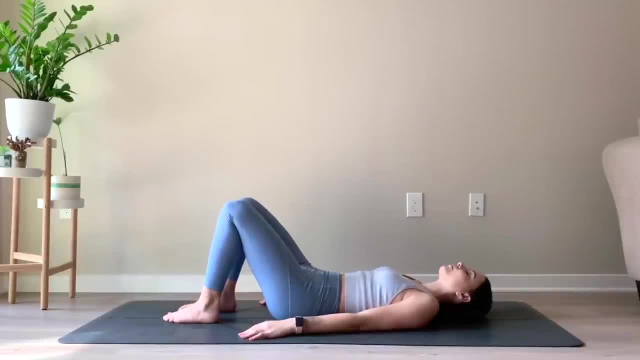 body, Coming into pigeon pose, keeping the left foot on the ground and crossing the right ankle on the left thigh just above the knee as you breathe in and out. Stay here if this is a deep enough hip stretch for you, or you can lift your left foot up. 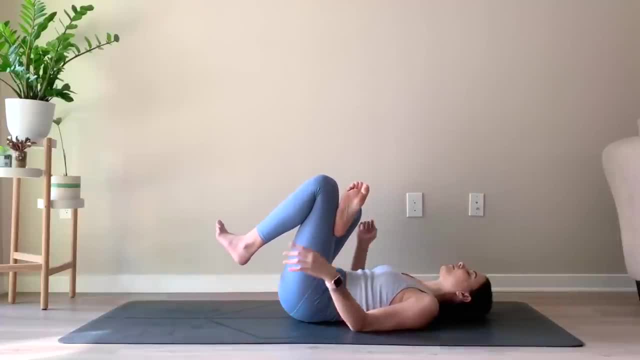 off the mat. bring your right arm in between your legs and interlace the fingers around the back of your left thigh, just behind the knee, Hugging your legs closer in towards your body getting a deeper stretch. Take one last breath here. 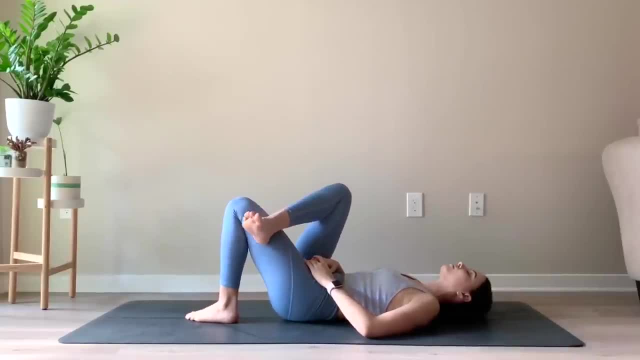 If your left foot is lifted, slowly, place it back down. Cross your right leg all the way over the left so that the right knee is over the left knee. Take a deep breath in, Take a deep breath out. Lift your right foot up off of the mat and place your hands on the tops of the feet. 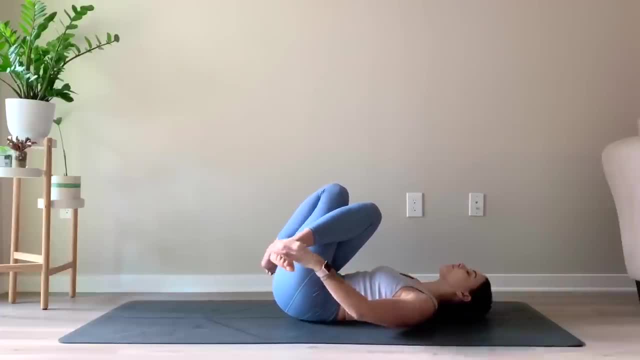 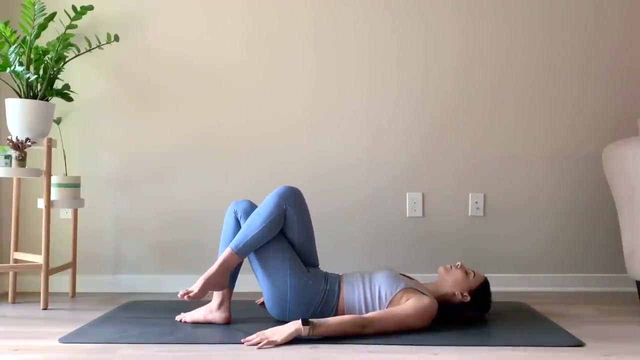 Drawing the heels towards your glutes, Getting a stretch in the right outer hip, Relaxing the shoulders, Maybe closing the eyes here. Take a deep breath in Placing your right foot back down and crossing the right leg over the left so both soles of the feet are flat on the ground. 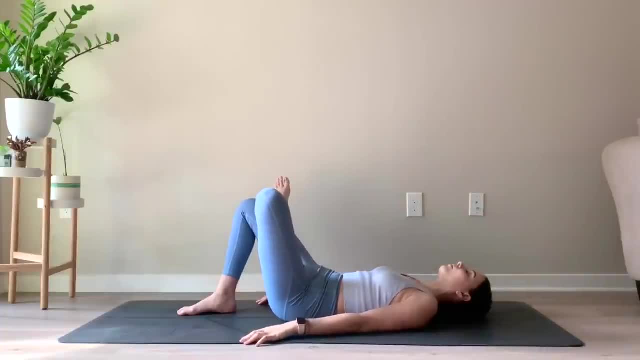 Keep your right foot planted down and cross your left ankle on top of your right thigh, just above your knee, Coming into our pigeon stretch, Choosing to stay here with your right foot on the ground, Gently pressing that left knee away from your body. 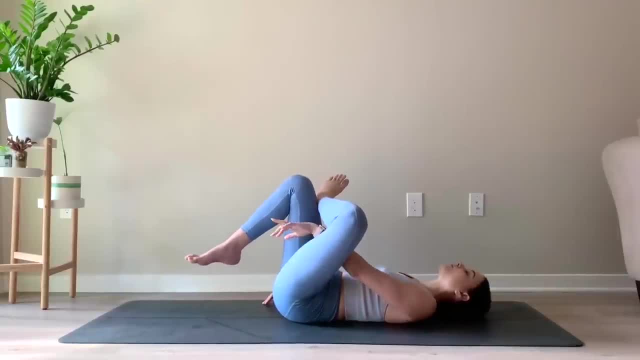 Or choosing to lift that right foot up, Bringing your left arm in between the legs, Interlacing the fingers, Placing them to the back of the right thigh And hugging both legs closer in towards your body, Keeping your left foot flexed. 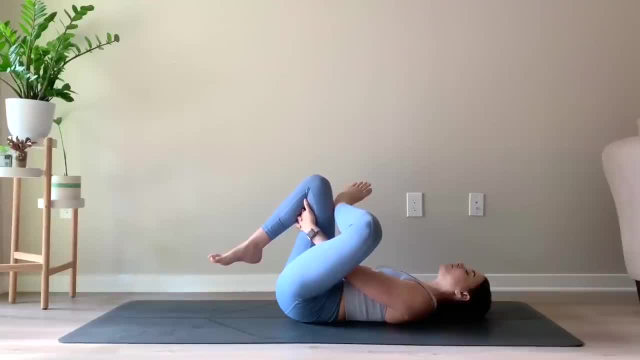 And coming back to your breath, Taking one more breath and if the right foot is lifted, go ahead and bring it back down. cross the left leg all the way over the right, so the left knee is stacked over the right knee, and then lift your right foot up off of the mats, place your hands to the tops of 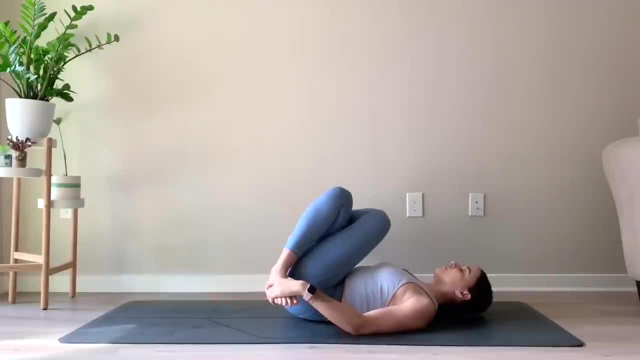 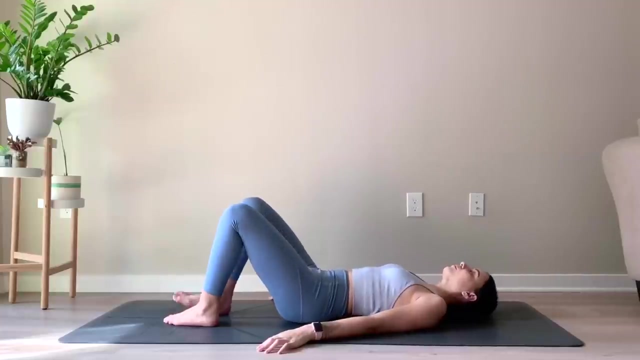 the feet, hugging the knees closer in towards your chest, letting the arms become heavy and breathing into that left hip. and with your next breath, gently release the grip on your feet. release the right foot back down and uncross the left leg and with your next breath, gently release the grip on your feet. 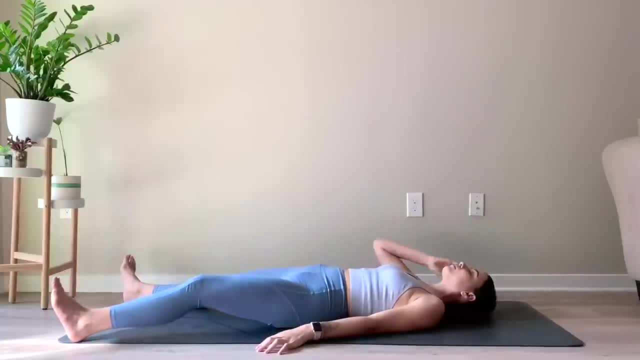 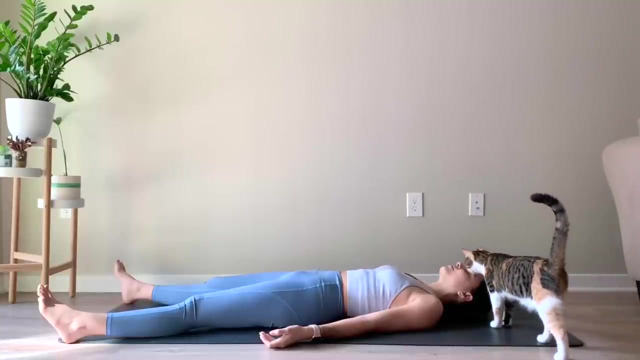 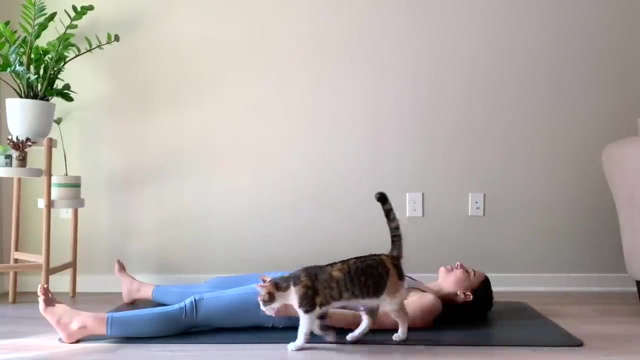 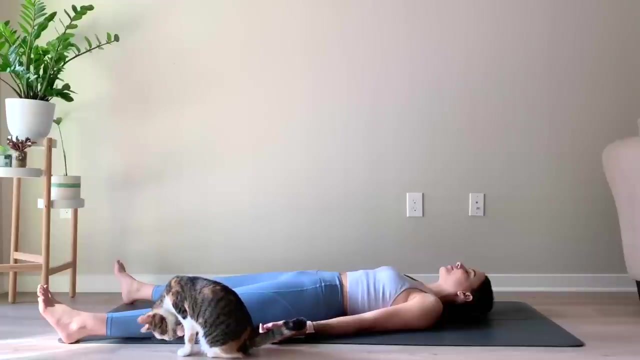 extend one leg at a time, straight out in front of you and allow the arms to rest alongside your body, with the palms face up, coming into our final resting pose. invite the eyes to close down and begin to bring your awareness to your physical body, just noticing how you feel here. 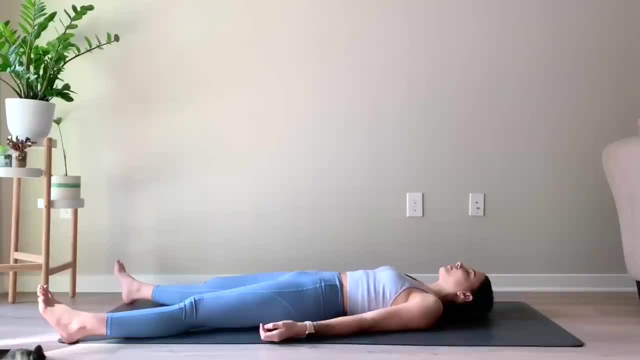 beginning to rest the feet, letting the legs become heavy, and begin to bring your awareness to your physical body. and begin to bring your awareness to your physical body, letting go of any tension. and the hips, the glutes- letting go of any tension. and the hips, the glutes. 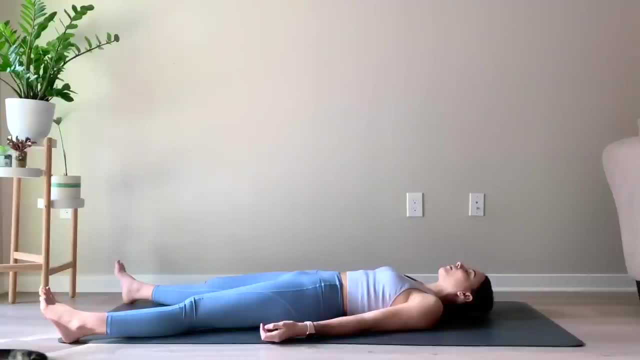 the glutes, the low back. notice how the belly and the chest move. the low back. notice how the belly and the chest move. you feel the expansion and the contraction of the belly like a miracle. Feel the shoulder blades pressed into the ground. Feel your face relax. 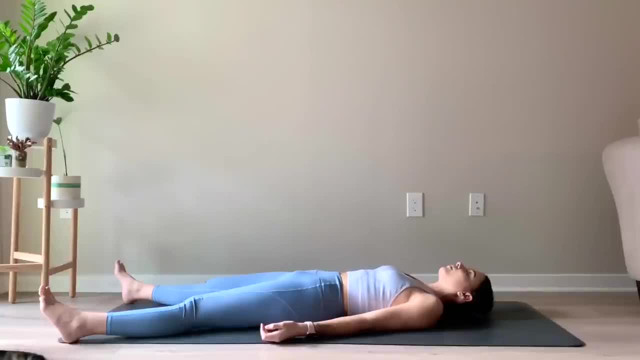 Unclench your jaw, Open the space in between the eyebrows, Feel your body relax all the way from the crown of your head down to the fingers and the toes. Relax And finding a cleansing breath here, Exhaling where you are. 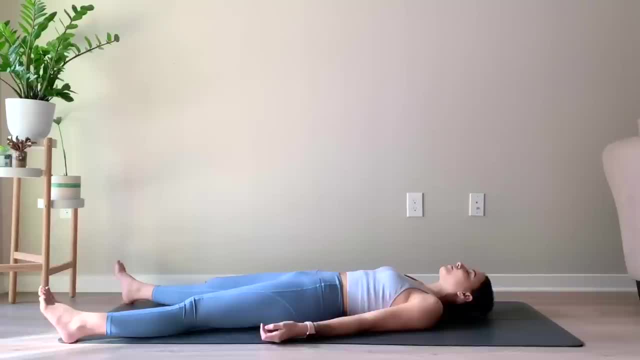 Take a big breath in through the nose, Open the mouth, Exhale out, Coming back, Exhaling, Exhaling, Exhaling, Exhaling, Exhaling, Exhaling. Welcome back to your natural rhythm of breath, as you start to wiggle the fingers and the 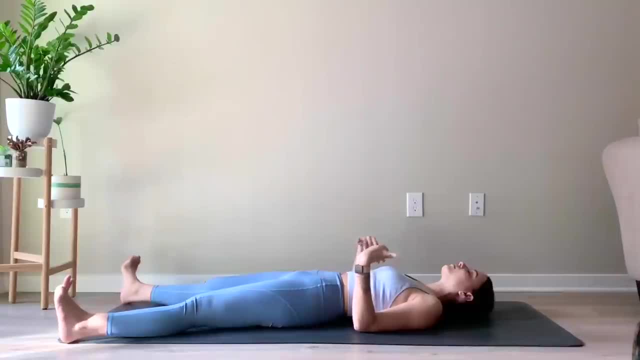 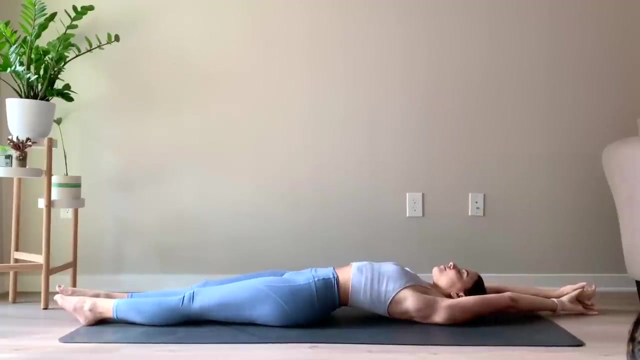 toes Start to awaken the body by rolling the wrists and rolling the ankles, Reaching the arms up overhead, Pointing the toes to the ground, Exhaling toes to find a full body stretch and gently bending the knees, placing your hands on top. 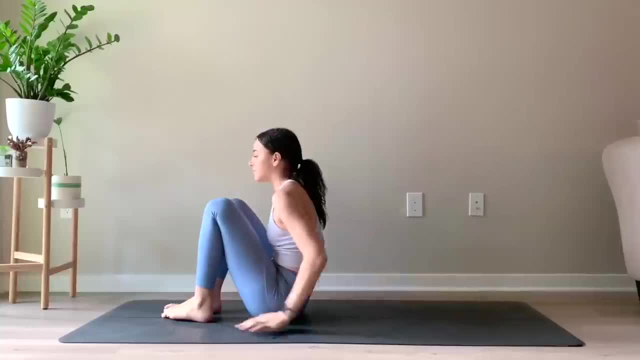 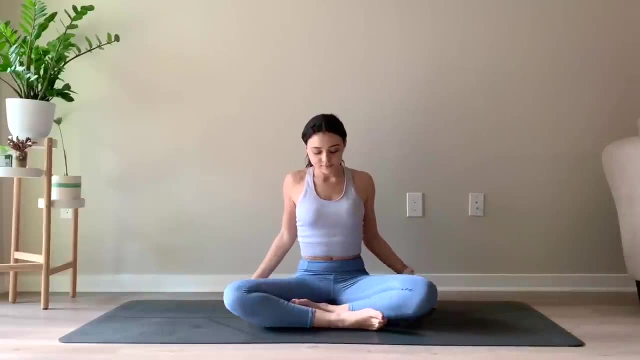 of the knees and very slowly rolling yourself up to come into a seated position, keeping your eyes closed or your gaze soft. rest your hands on top of your legs and come back to your breath, taking a moment to find gratitude for yourself for coming on your mat today.